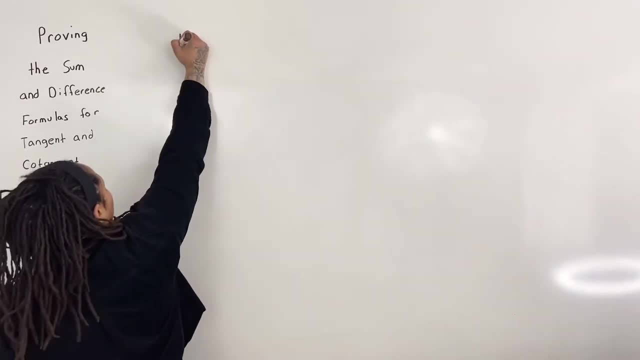 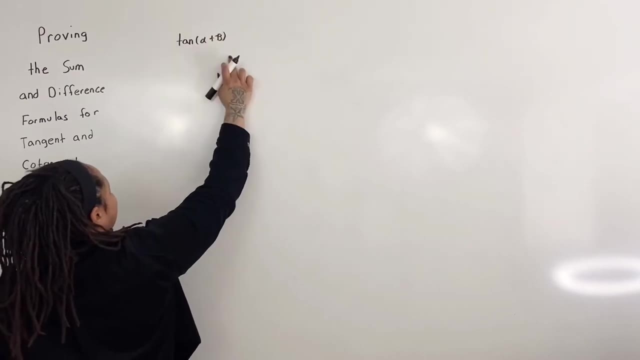 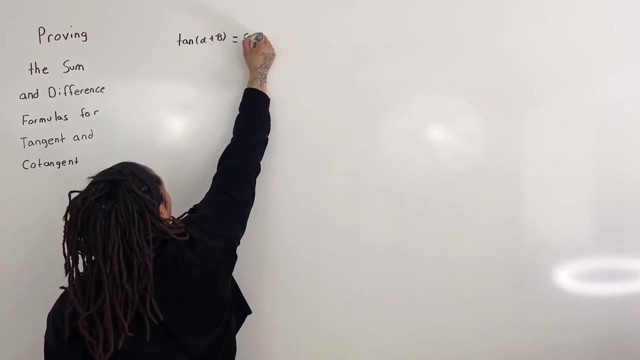 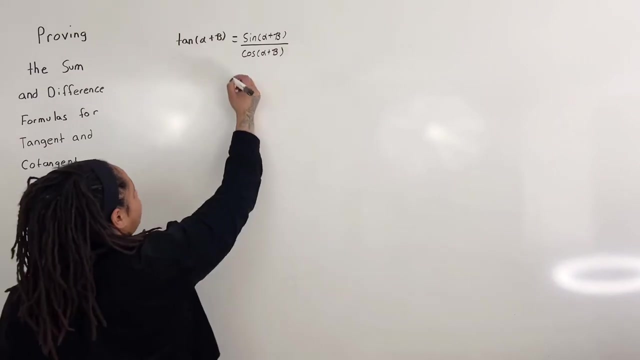 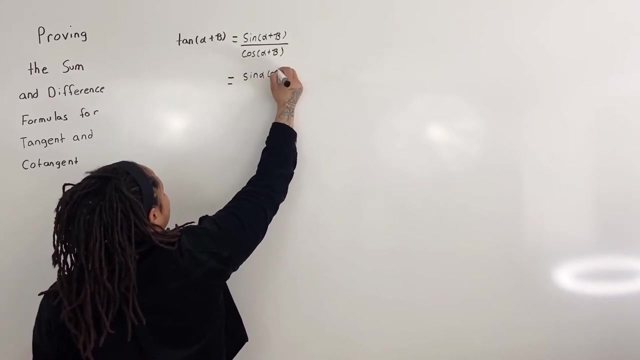 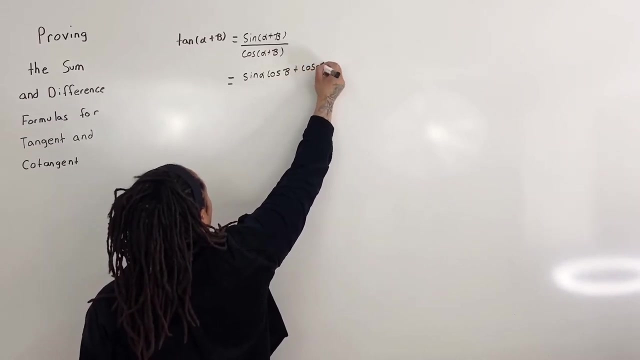 beta. So we say tangent of alpha plus beta and we know by our quotient identity that tangent of alpha plus beta is equal to sine of alpha plus beta over cosine of alpha plus beta, and by the sum formula for sine we have sine of alpha, cosine of beta plus cosine of alpha. 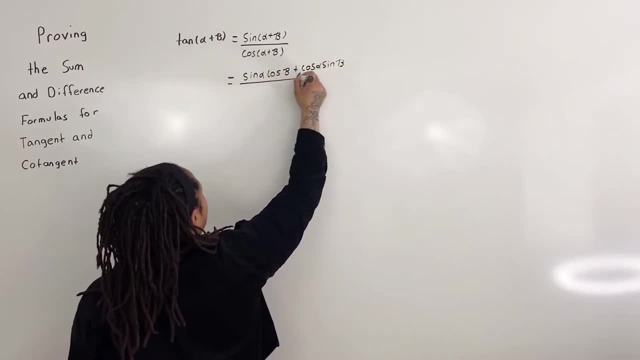 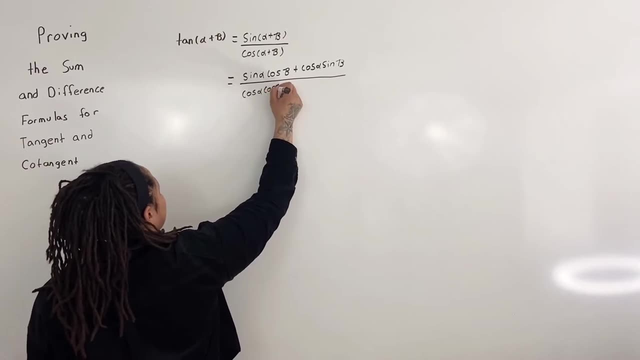 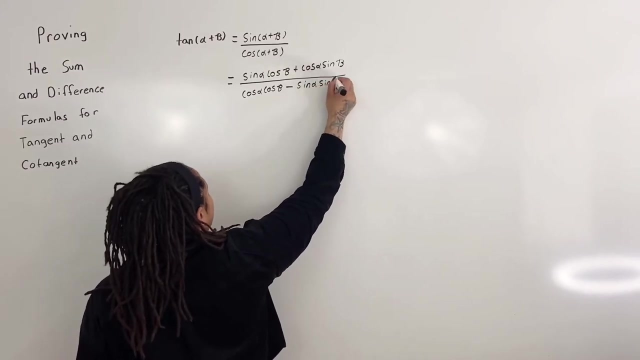 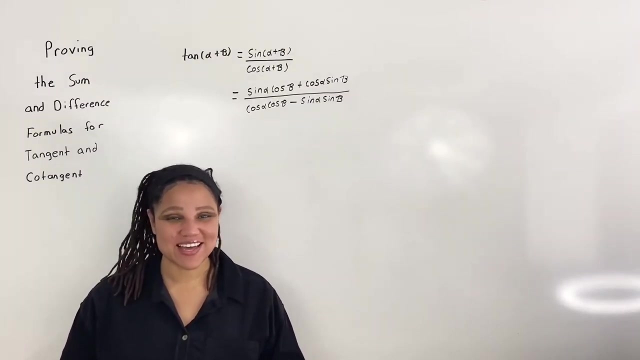 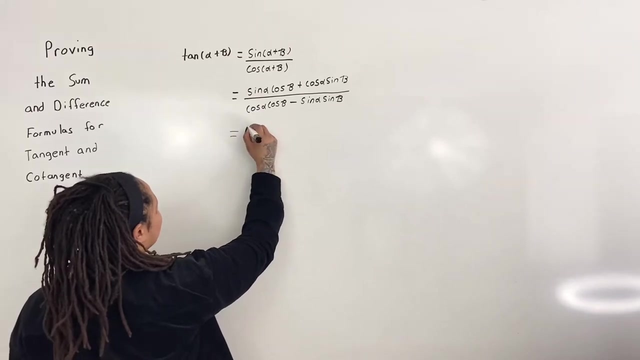 sine of beta, and by the sum formula for cosine, we have cosine of alpha cosine of beta, minus sine of alpha sine of beta. Now I'm going to multiply the numerator and the denominator by cosine of alpha cosine of beta. So we're going to say that all this is equal to sine of alpha cosine. 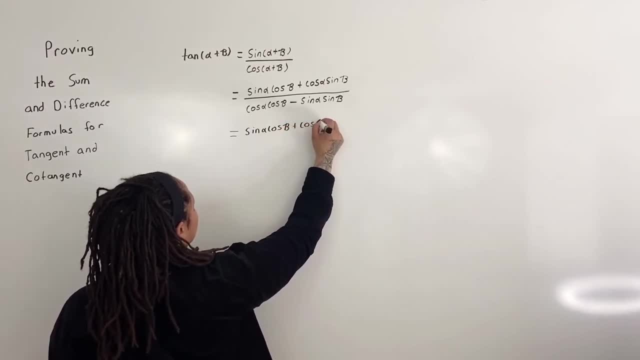 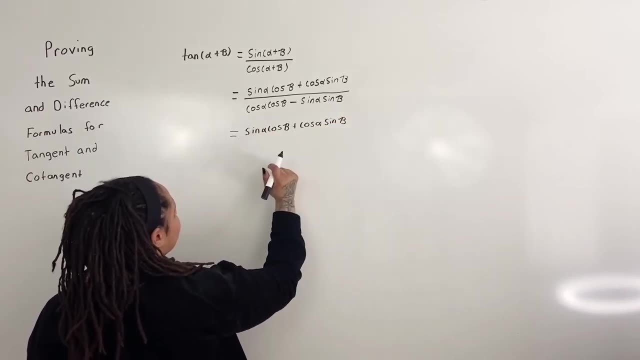 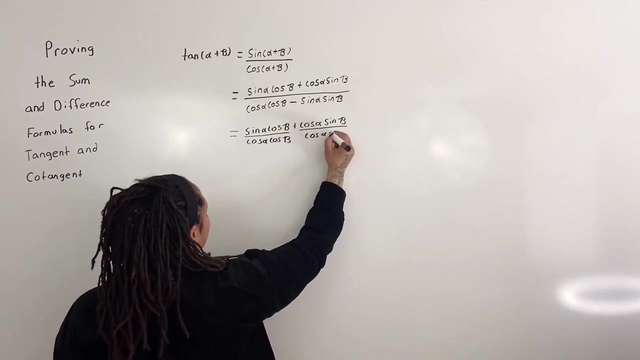 of beta plus cosine of alpha, sine of beta. And now in the numerator I'm going to divide everything through by cosine of alpha, cosine of beta. So we have cosine of alpha, cosine of beta, And here we have cosine of alpha, cosine of beta. And now we need to do the exact. 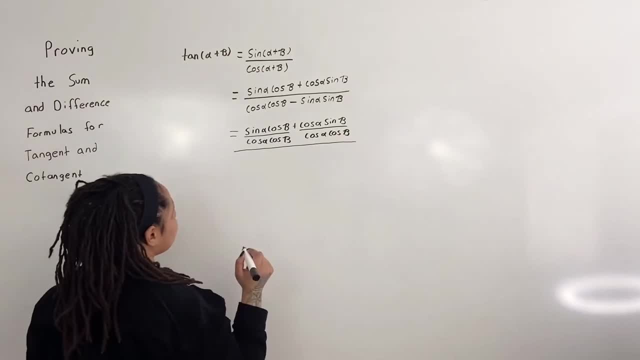 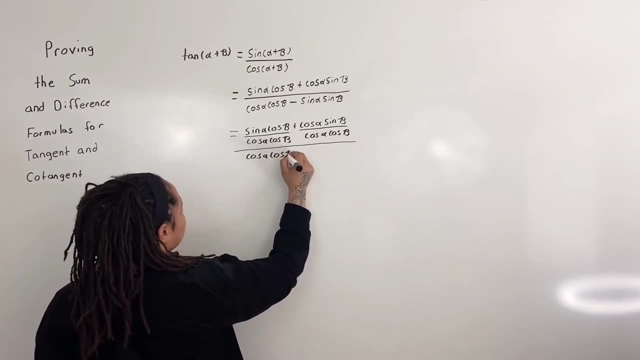 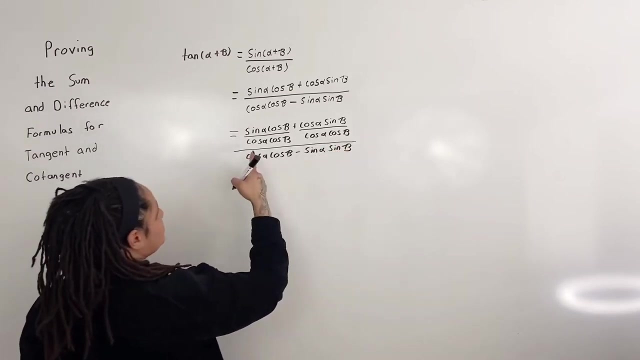 same thing in the denominator. So I'm going to rewrite the denominator. We have cosine of alpha, cosine of beta, minus sine of alpha, sine of beta, And now I'm going to divide everything through by cosine of alpha, sine of beta. And here we have cosine of alpha, cosine of. 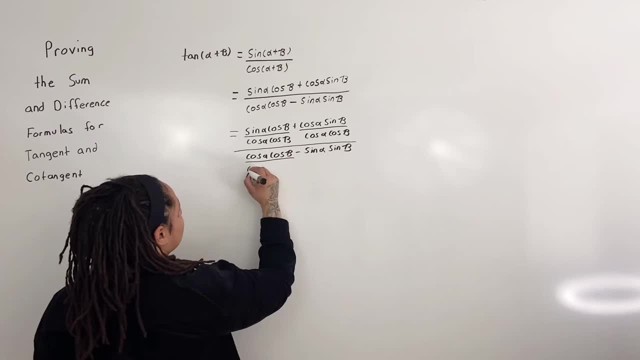 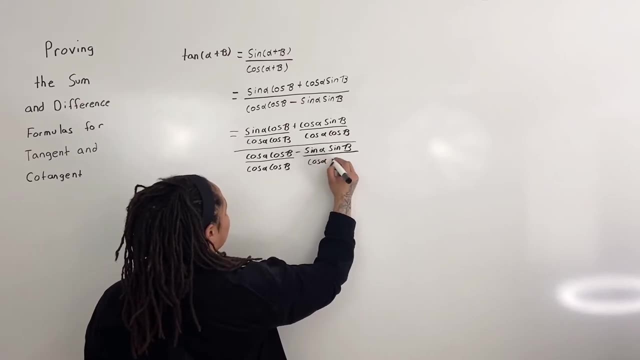 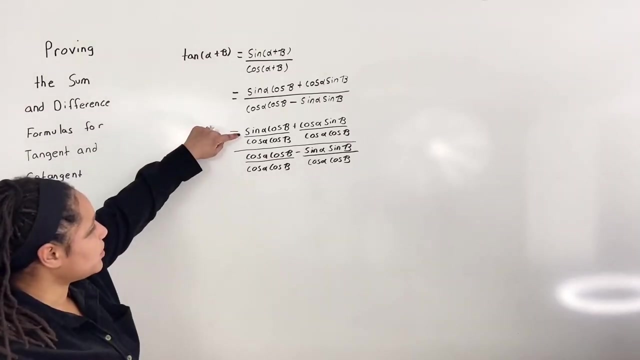 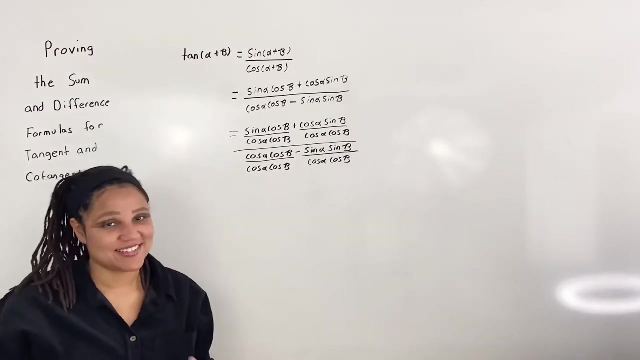 beta. So here we have cosine of alpha, cosine of beta, And here we have cosine of alpha, cosine of beta. Now we see that by the quotient identity sine of alpha divided by cosine of alpha is tangent of alpha. So I'm going to say: 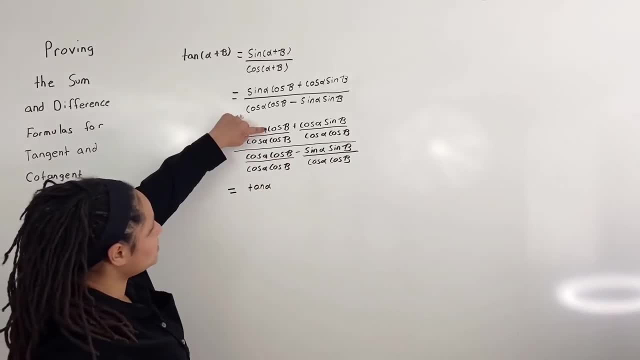 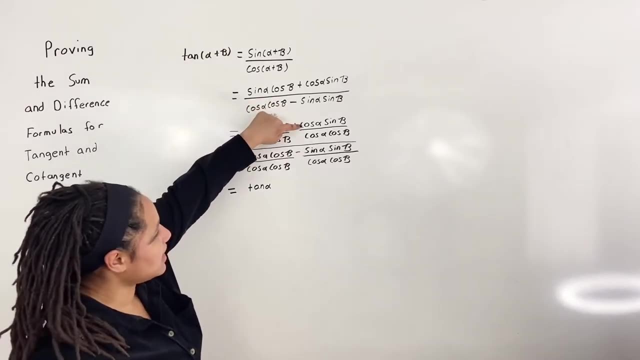 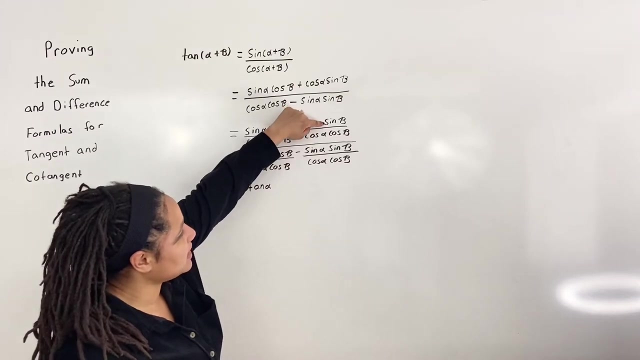 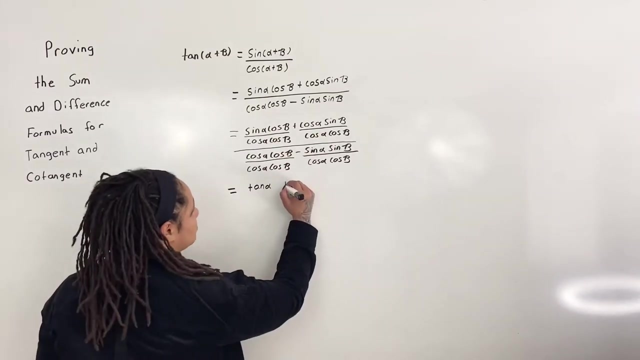 tangent of alpha And I see that cosine of beta divided by cosine of beta is just one. And I see that cosine of alpha divided by cosine of alpha is just one. And here we have sine of beta divided by cosine of beta, which is tangent of beta. So we have plus tangent of beta. 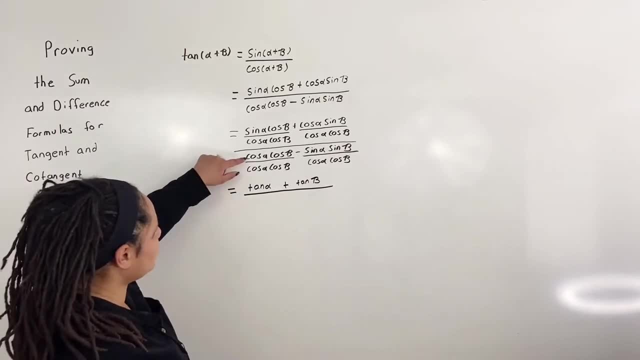 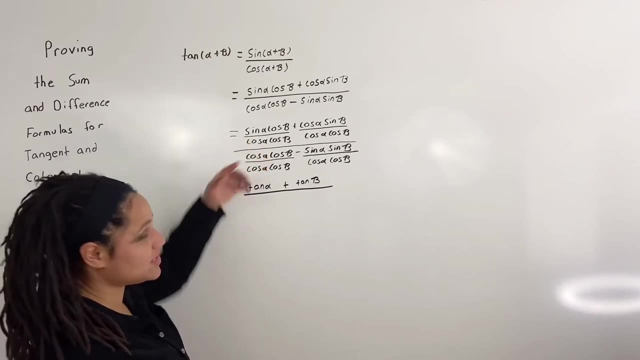 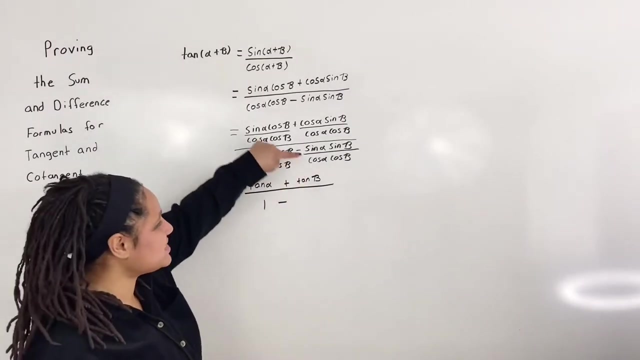 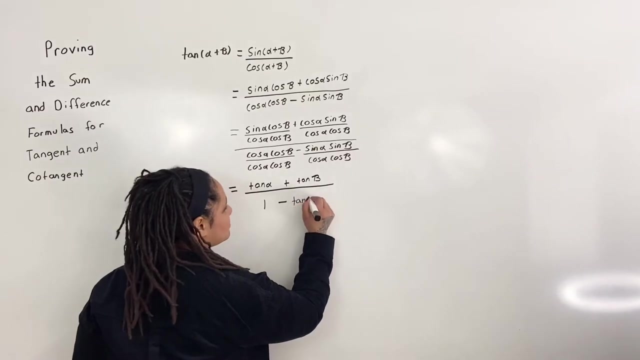 Now in the denominator we see that cosine of alpha divided by cosine of alpha is one, And cosine of beta divided by cosine of beta is one. So here I can just put one minus. And here we have: sine of alpha divided by cosine of alpha is tangent of alpha, And sine of beta divided by cosine of beta. 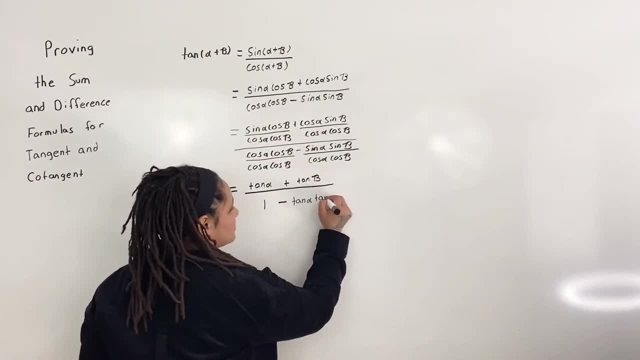 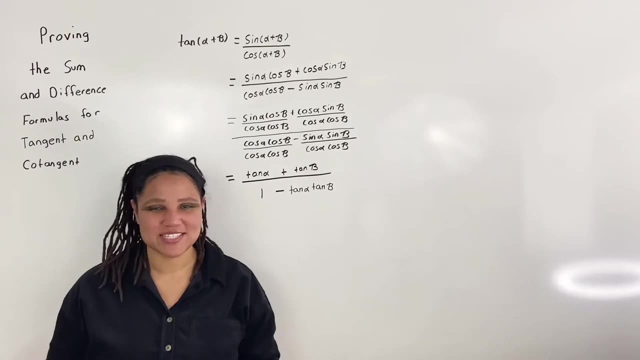 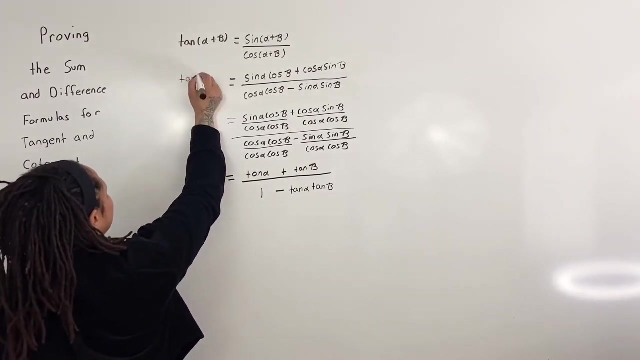 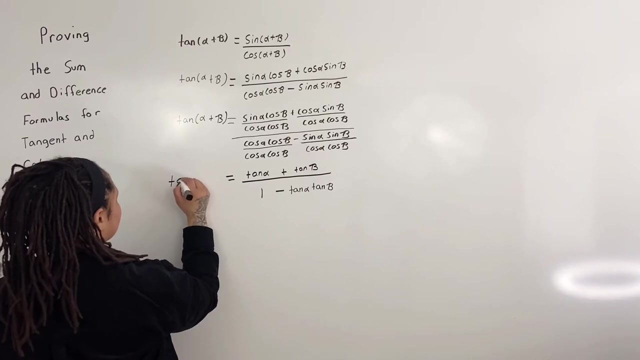 is tangent of beta. And now I'm just going to bring everything down on the left side of the equation so we can see the sum formula for tangent. So we have tangent of alpha plus beta, and here we have tangent of alpha plus beta. and here we have tangent of alpha plus beta. 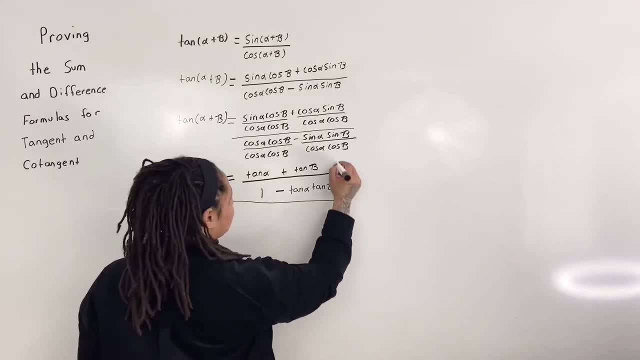 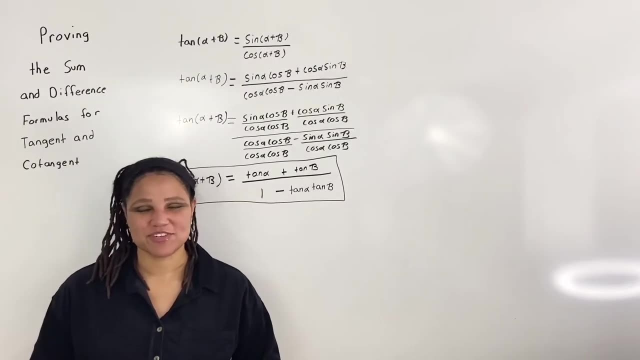 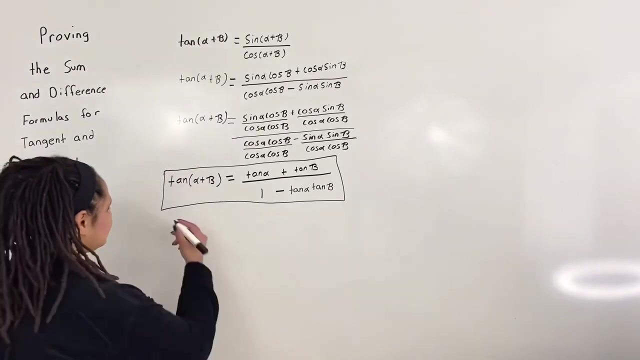 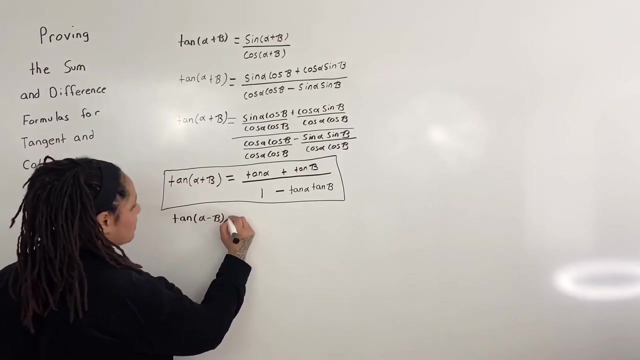 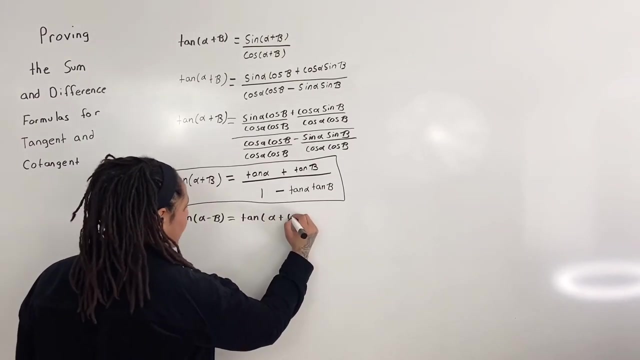 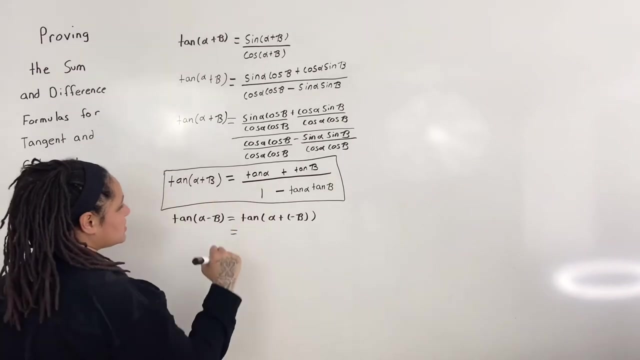 And here is our sum formula for tangent. Now we will use the sum formula for tangent to come up with the difference formula for tangent. So we have: tangent of alpha minus beta is equal to tangent of alpha plus a negative beta, which is equal to. now we're going to use the sum formula for tangent. so we have: 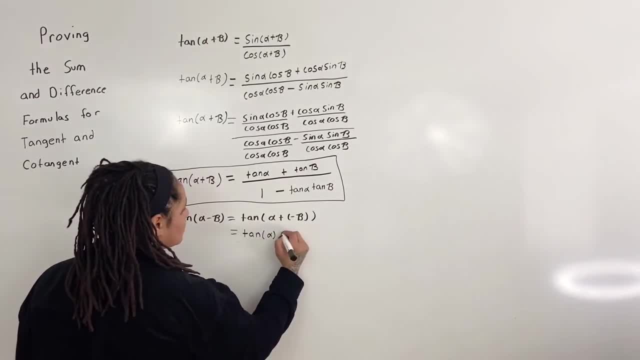 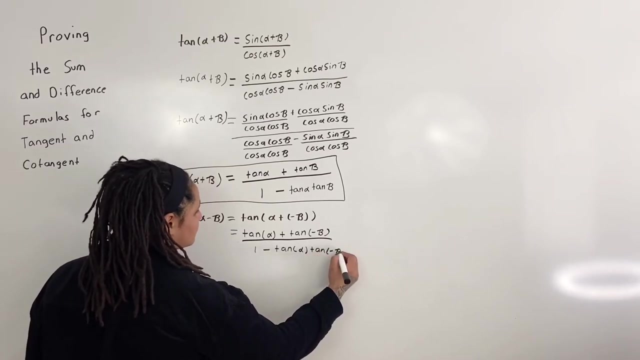 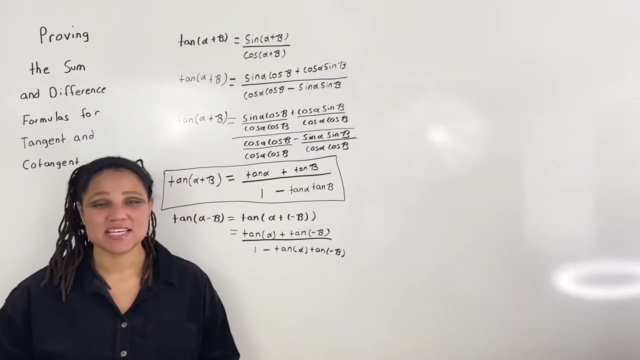 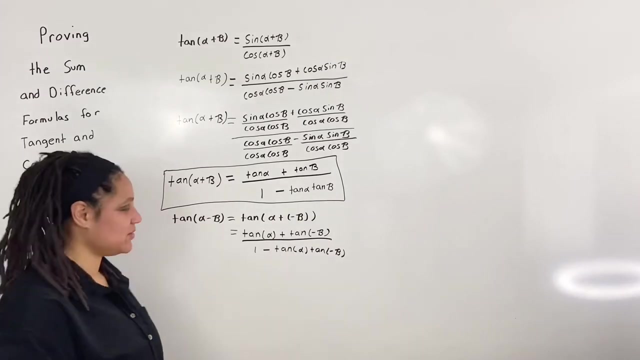 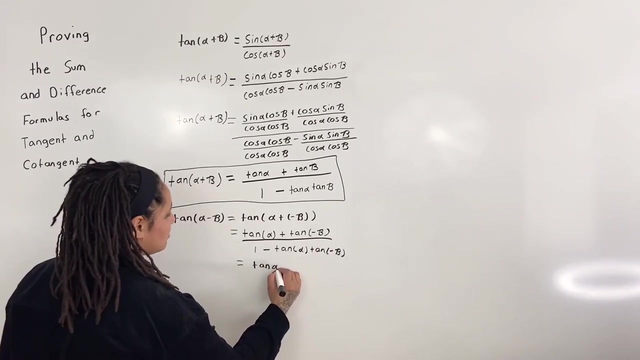 tangent of alpha plus tangent of negative beta all over one minus tangent of alpha times tangent of negative beta. Now we know that tangent is an odd function. this means that we can take the negative sign and pull it out of the function. so that's what we're going to do. so we have. this is equal to tangent of alpha minus. 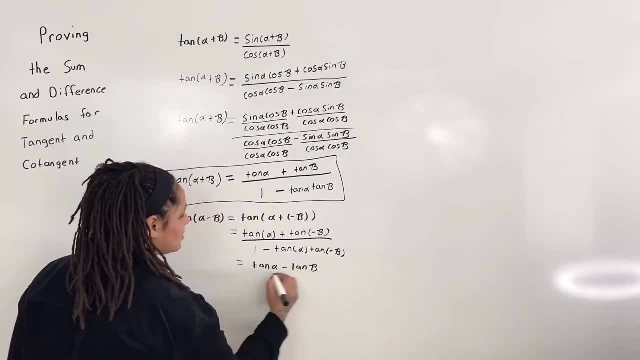 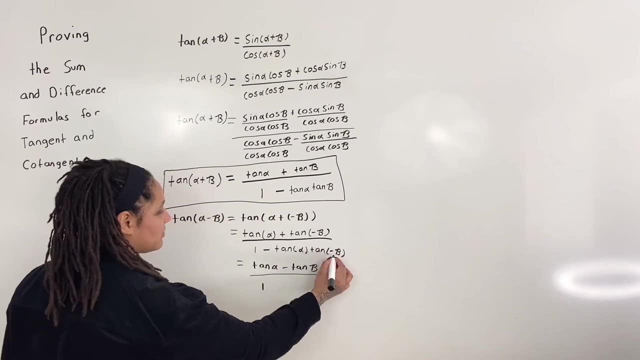 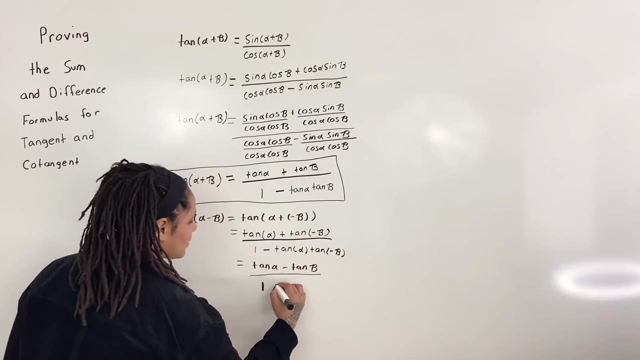 tangent of beta all over one and this negative sign will come out of the function and it will make this negative sign become positive. so we have one plus tangent of alpha, tangent of beta, and now I'm just going to bring the left side all the way down. 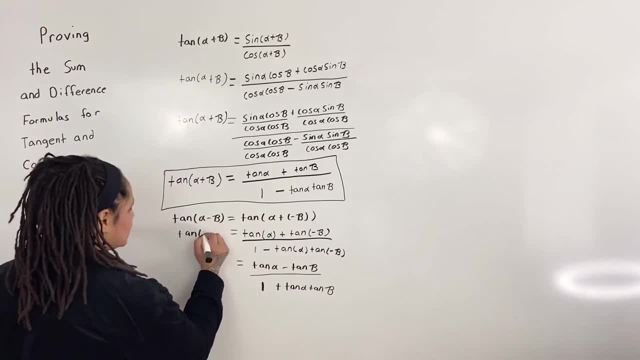 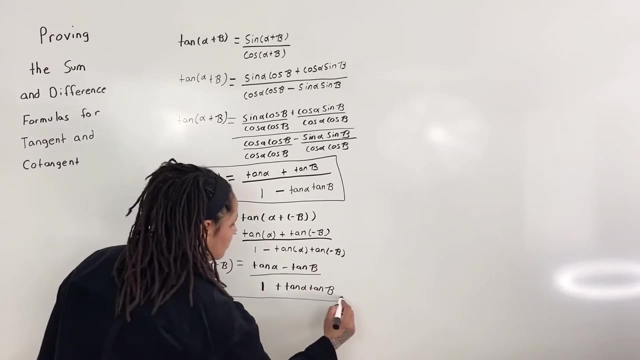 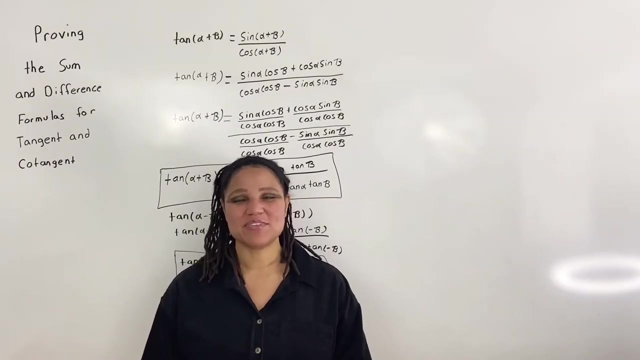 so here we have tangent of alpha minus beta, and here we have tangent of alpha minus beta, and now we have the difference formula for tangent. now we are going to prove the sum formula for cotangent. we begin with cotangent of beta and then we say that the negative sign must be equal to the negative sign of. 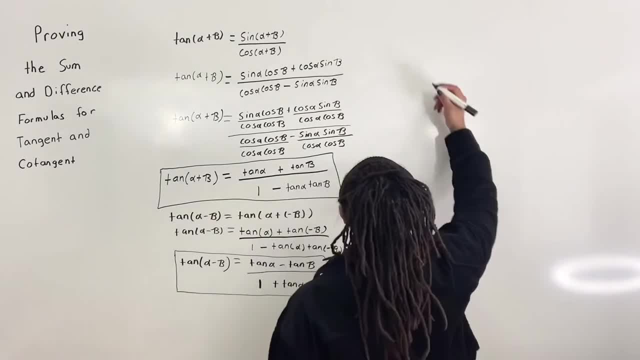 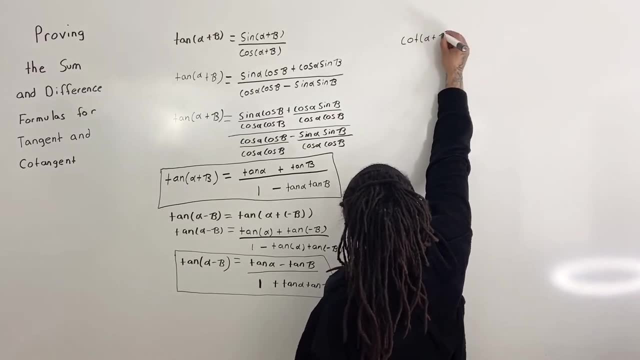 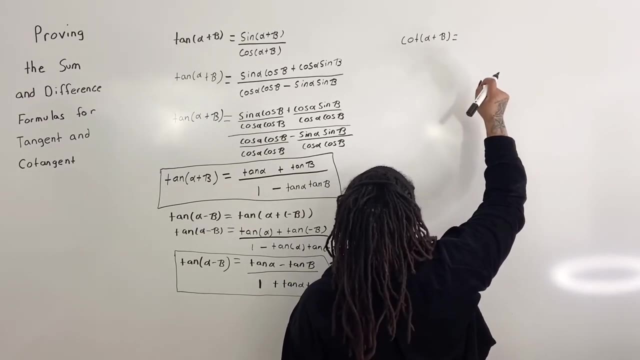 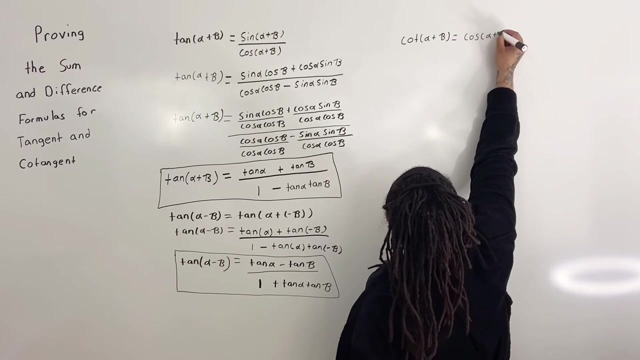 alpha plus beta. so we say: cotangent of alpha plus beta is equal to- and we're going to rewrite it in terms of cosine and sine. so we have cosine of alpha plus beta divided by sine of alpha plus beta, and now we're going to apply the sum. 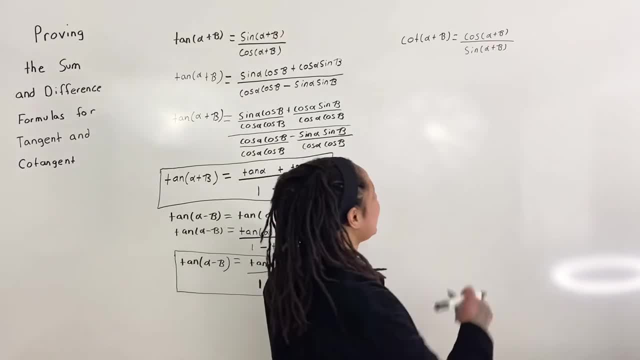 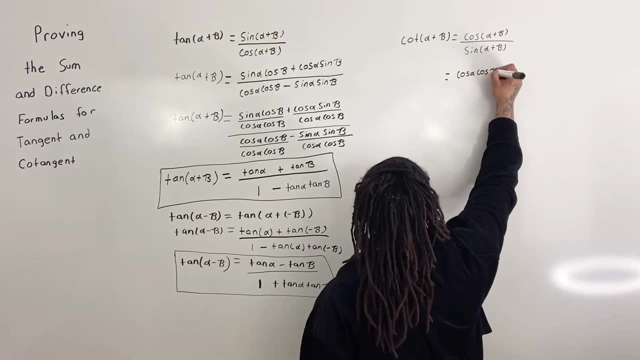 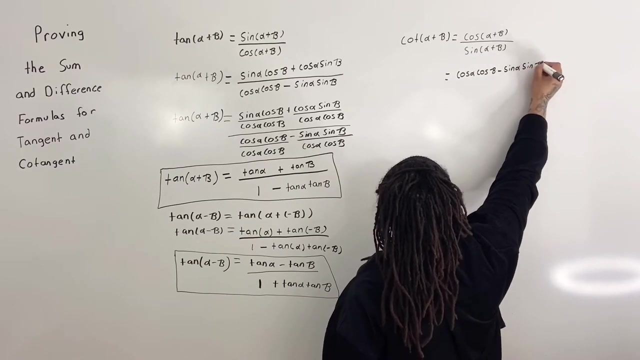 formula for sine and cosine. so we have: this is equal to cosine of alpha, cosine of beta minus, sine of alpha, sine of beta. all of this from the channel of sine and cosine, and sine of beta plus beta plus the integral of cosine, of alpha, cosine and cosine of beta. all of this from the 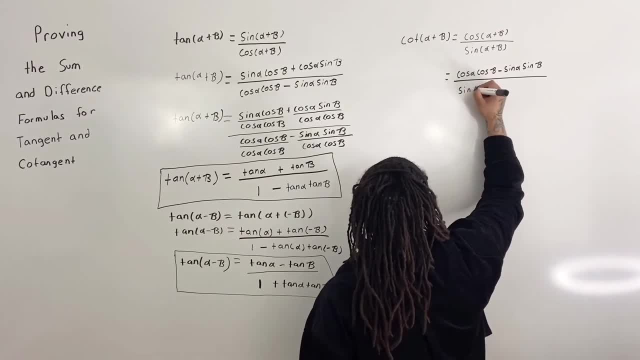 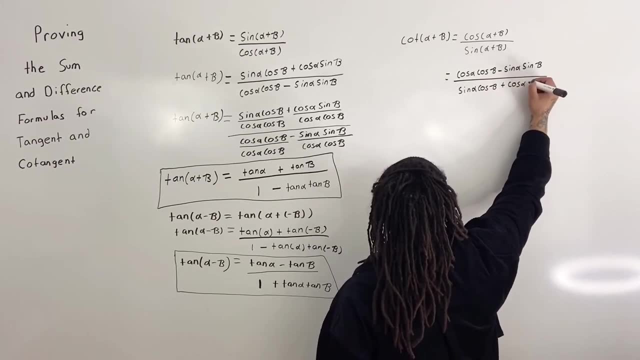 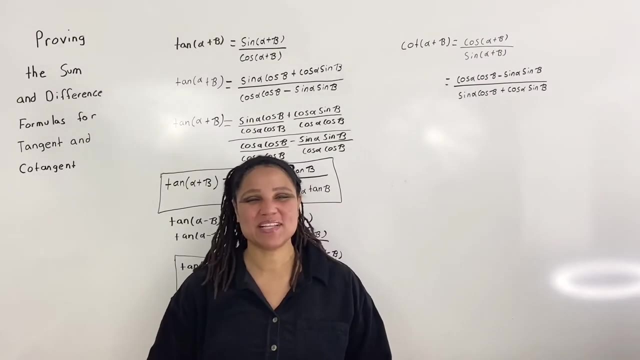 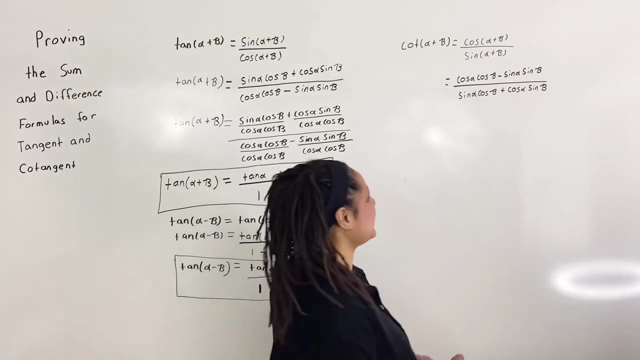 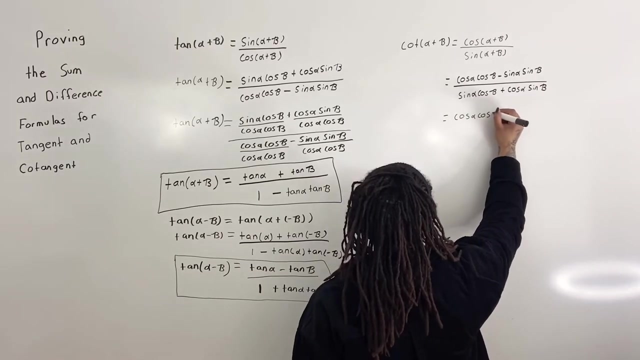 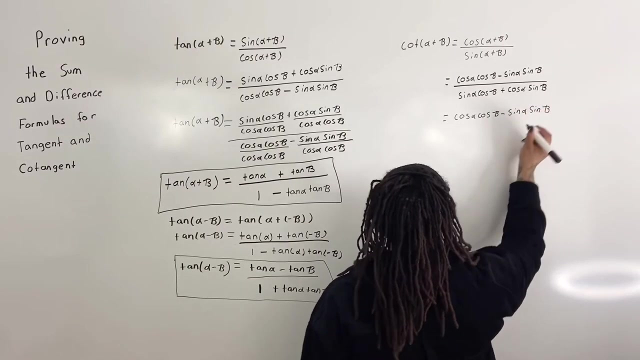 over sine of alpha cosine of beta plus cosine of alpha sine of beta. And now we're going to multiply the numerator and the denominator by sine of alpha sine of beta. So we're going to say this is equal to cosine of alpha cosine of beta minus sine of alpha sine of beta. And now I'm 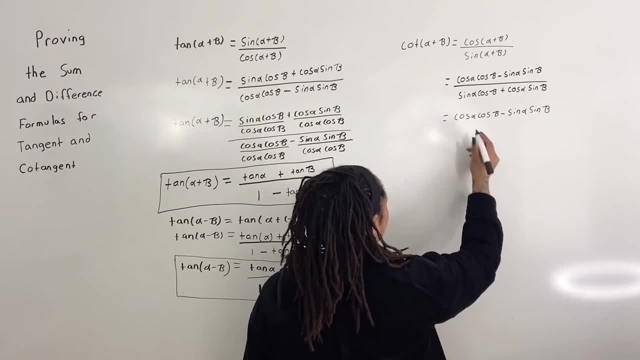 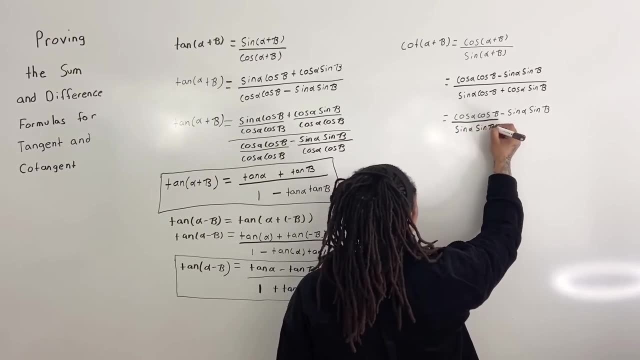 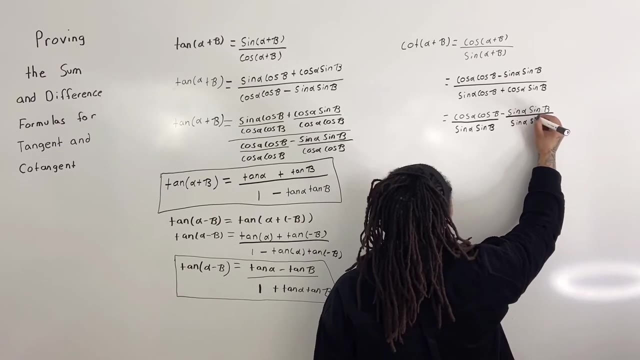 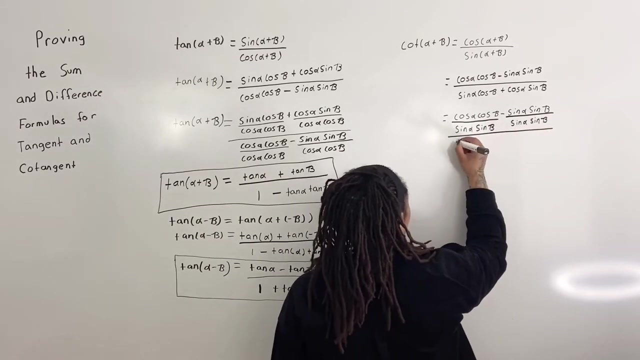 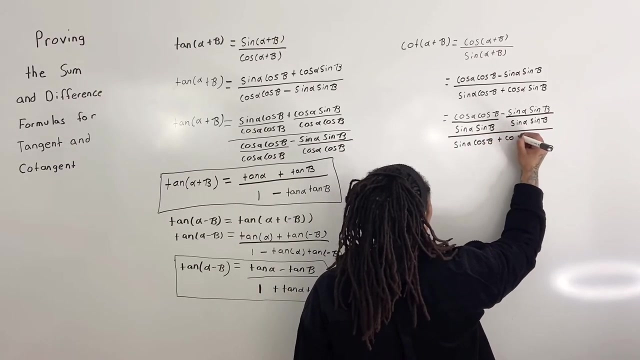 going to divide through by sine of alpha sine of beta. So we have sine of alpha sine of beta, And here we have divided by sine of alpha sine of beta, And now I'm just going to rewrite the denominator. So we have sine of alpha cosine of beta plus cosine of alpha sine of beta, And I'm going to 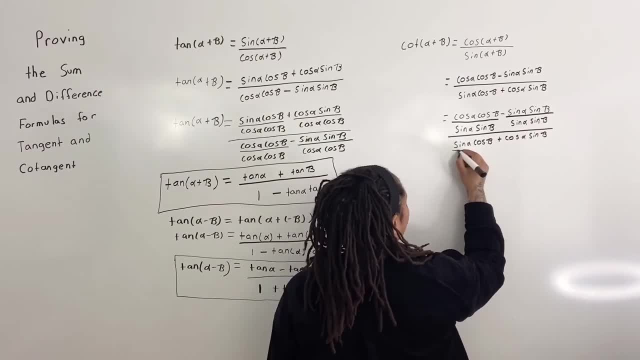 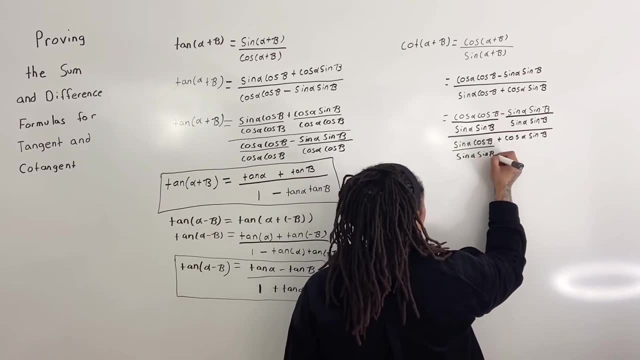 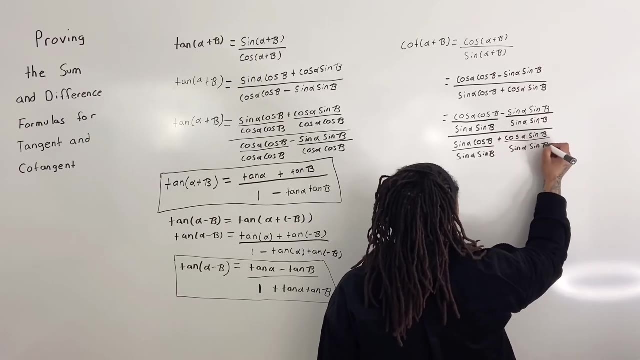 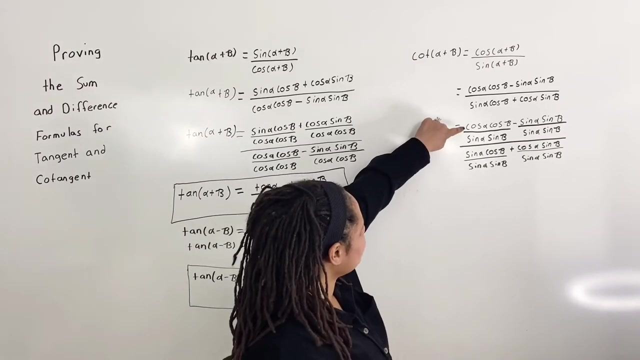 divide through by sine of alpha, sine of beta. So we have divided by sine of alpha, sine of beta, And here we have divided by sine of alpha, sine of beta. Now we are ready to simplify. Here we see that cosine of alpha divided by sine of alpha is: 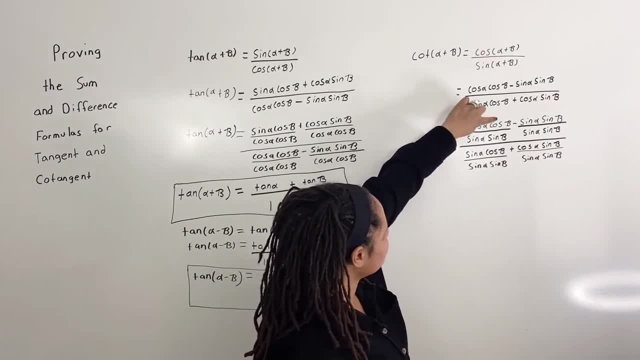 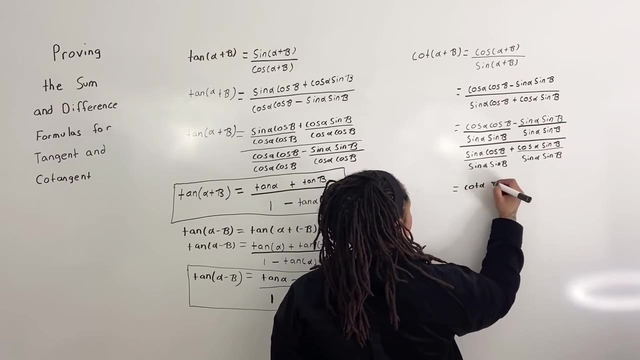 cotangent of alpha And cosine of beta divided by sine of beta is cotangent of beta. So I'm going to say this is equal to cotangent of alpha, cotangent of beta minus. and here we have sine of alpha, sine of beta divided by 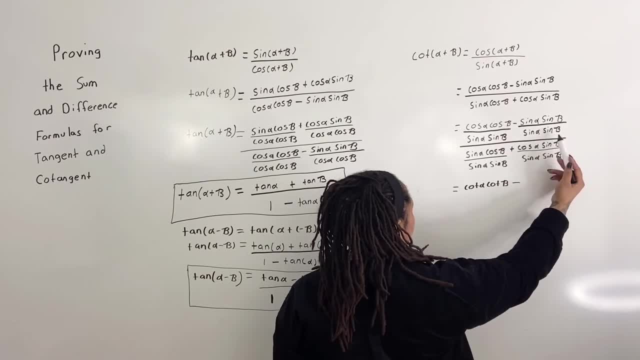 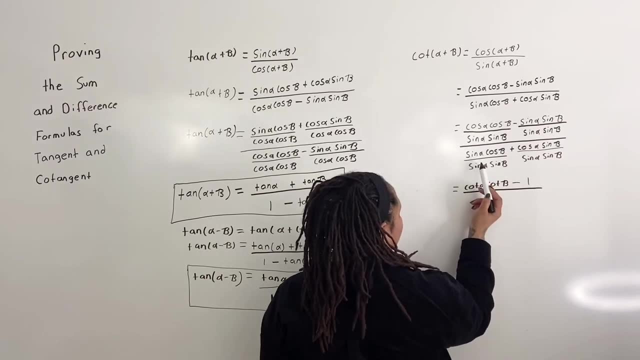 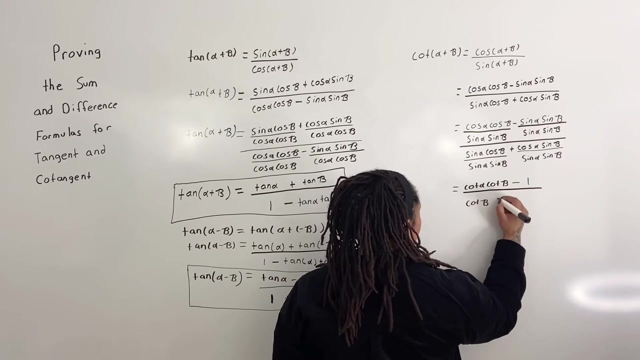 sine of alpha, sine of beta, which is equal to one divided by sine of alpha, divided by sine of alpha is just one, And cosine of beta divided by sine of beta is cotangent of beta. So we have cotangent of beta plus. here we have cosine of alpha divided by sine. 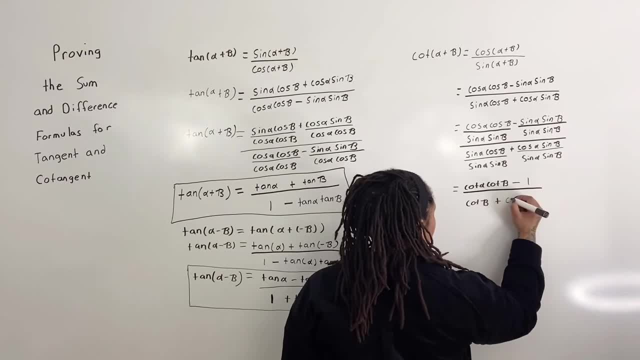 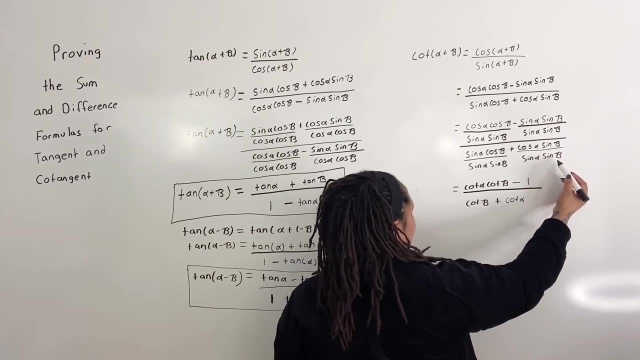 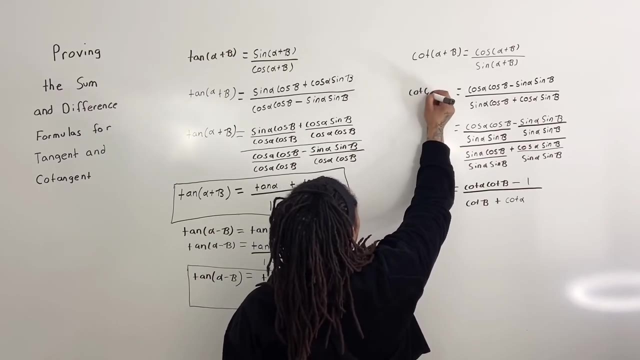 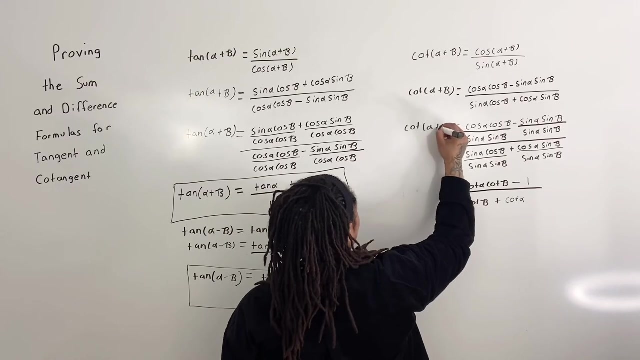 of alpha, which is cotangent of alpha, And here we have sine of beta divided by sine beta, which is just 1.. So now I'm going to just bring down everything on the left-hand side. So we have cotangent of alpha plus beta, Here we have cotangent of alpha plus beta, And here we have. 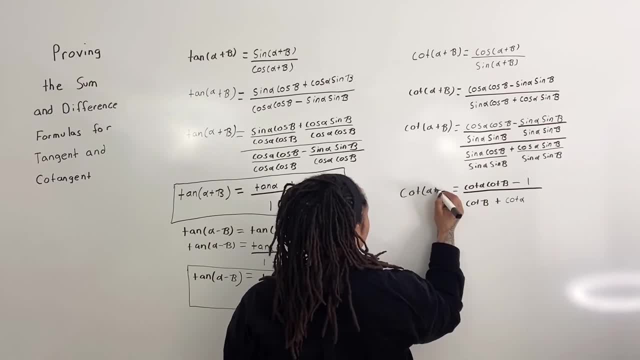 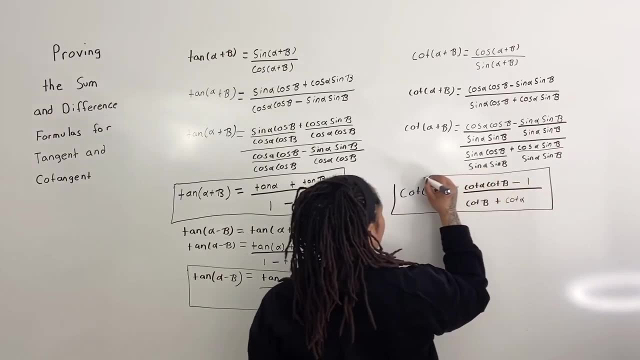 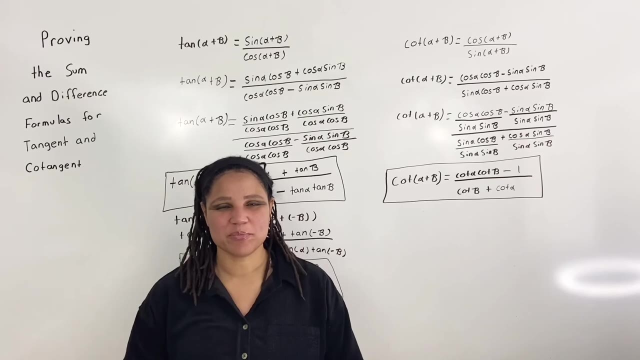 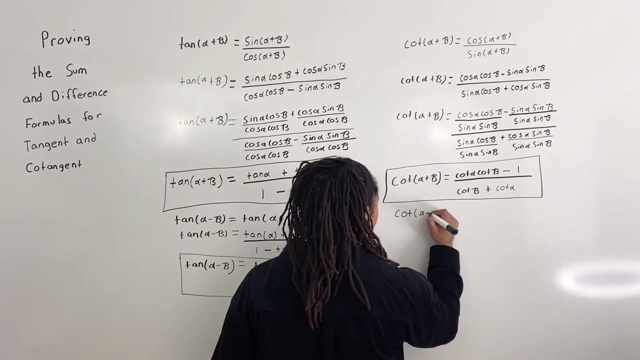 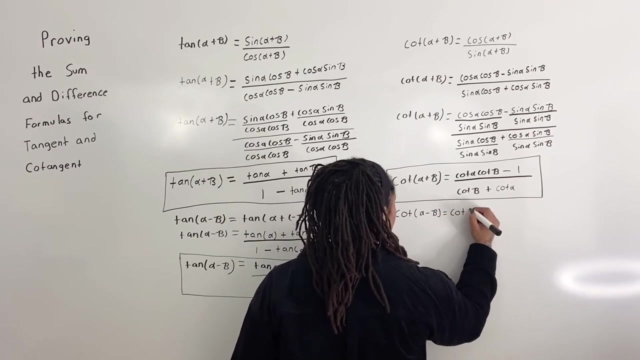 cotangent of alpha plus beta. And here is our sum formula for cotangent. And now we are going to use the sum formula for cotangent to come up with the difference formula for cotangent. So here we have: cotangent of alpha minus beta is equal to cotangent of alpha plus a negative beta, which is equal to, and now 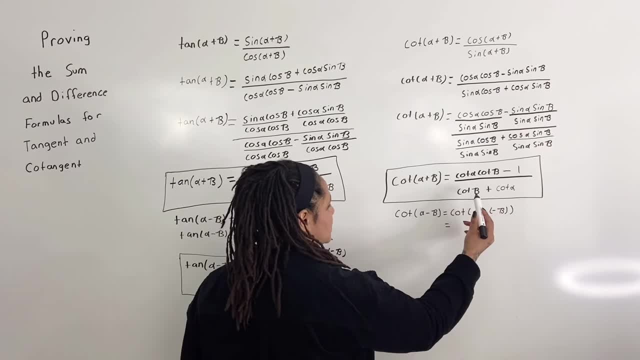 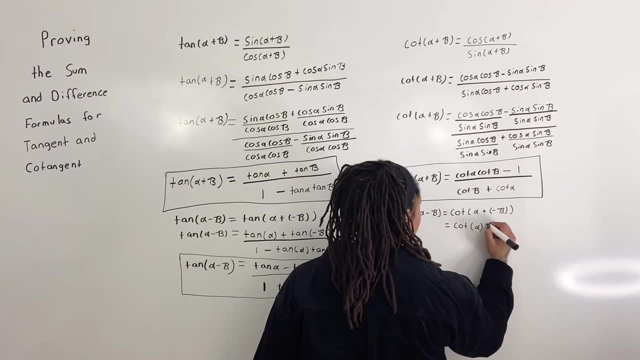 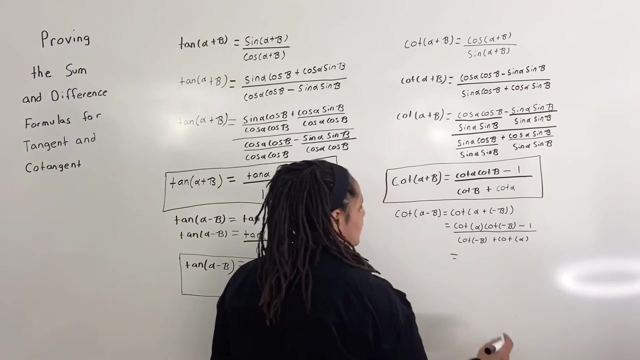 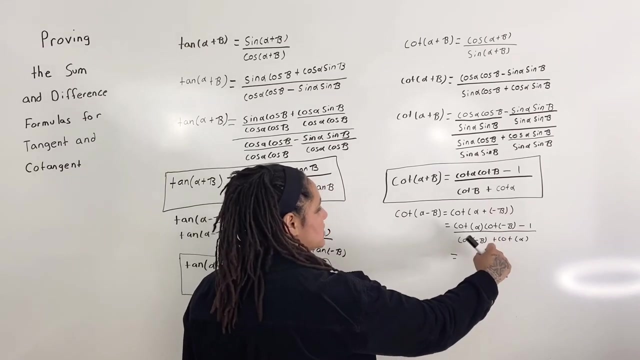 I'm going to add the sum formula for cotangent. So we have cotangent of alpha, cotangent of negative beta minus 1 divided by cotangent of negative beta plus cotangent of alpha, which is equal to. and now we're going to apply the odd identity for cotangent. We know that cotangent is an odd function, so we 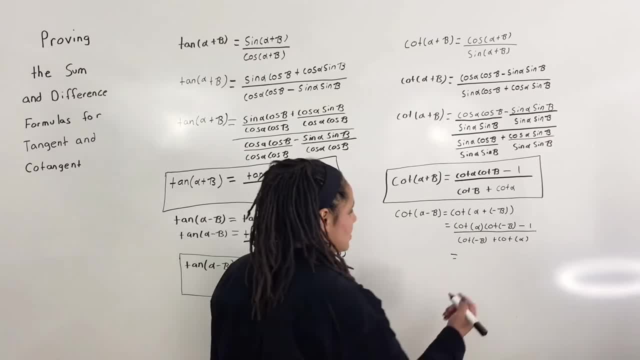 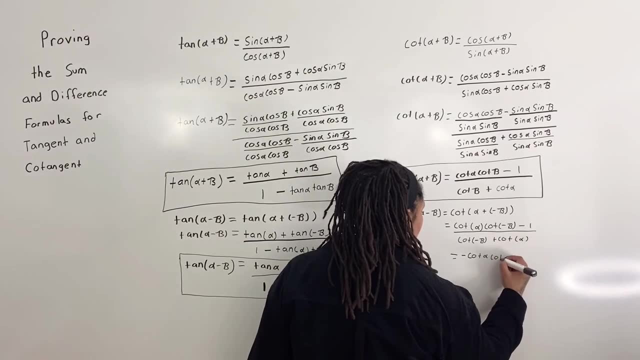 can simply pull it out. And here we have cotangent of alpha plus beta. And here we have cotangent of alpha plus beta, And here we have cotangent of alpha plus a negative beta, And we're going to pull out the negative sign. So we have negative cotangent alpha cotangent beta minus 1 divided by, and we're